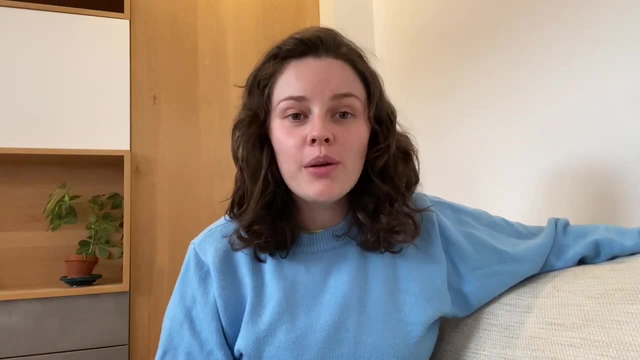 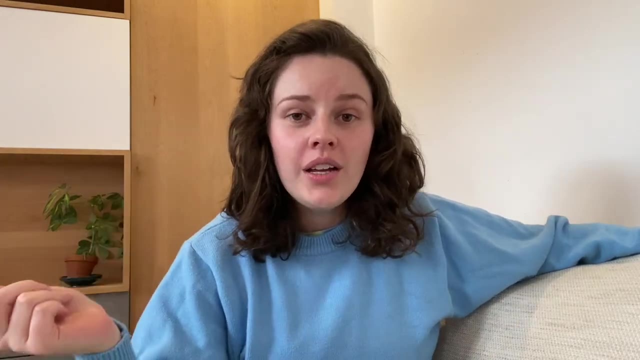 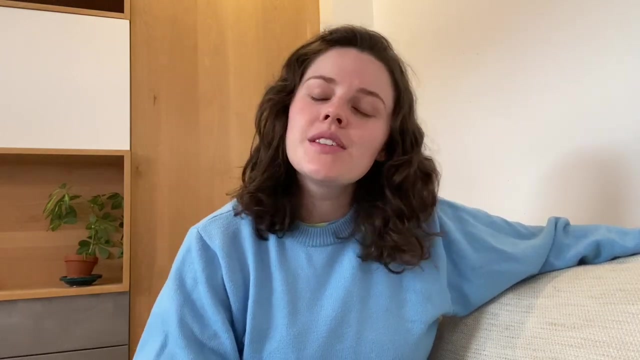 pour a cup of tea in the morning or sit on the couch. it's not about that. it's about actually understanding the job. So this video is very much for somebody who's looking to start the software engineering career and who really just has no idea what we do. This video is also 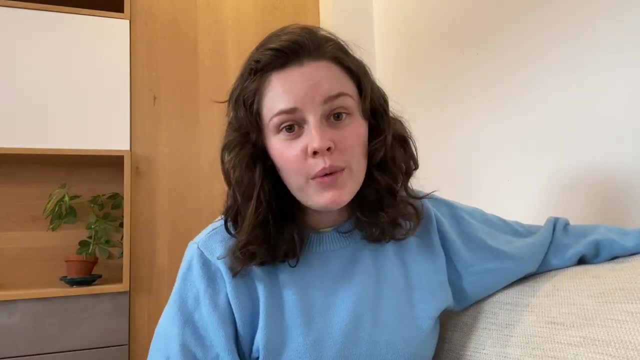 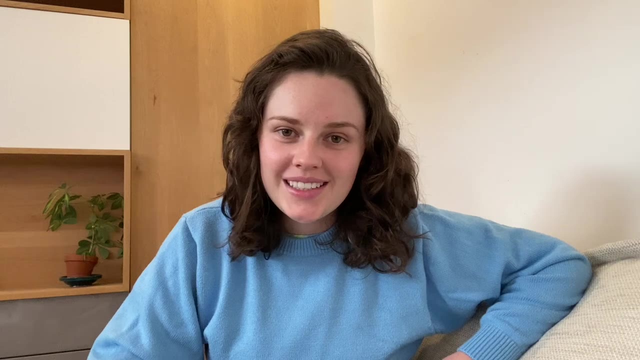 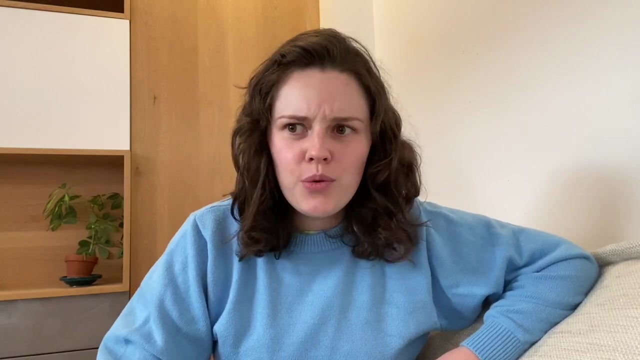 for people like my parents, who also have no idea what we do, no matter how many times I explain it to them. ур explanation i will take you through today is very much the same sort of explanation i tell any friend or family member, so it's very, very simplified for anyone to understand, not just somebody who's 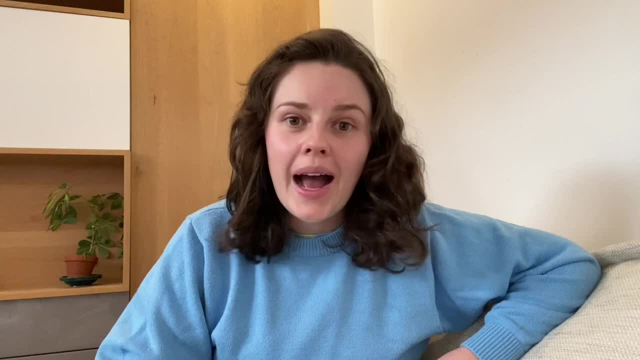 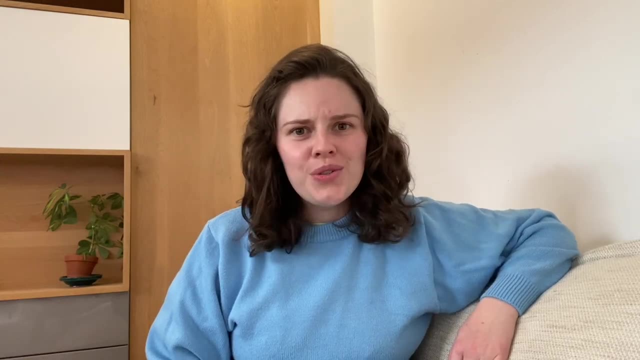 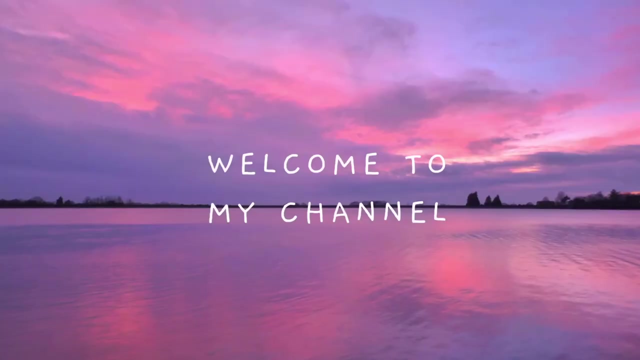 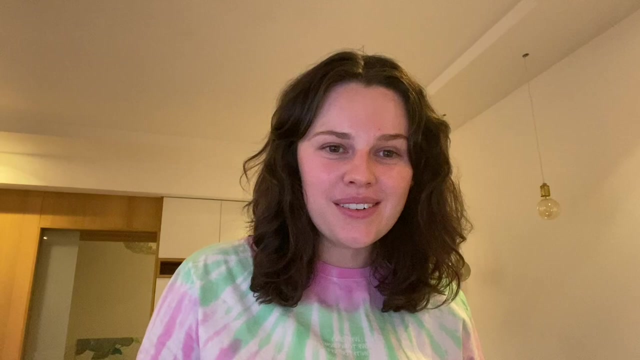 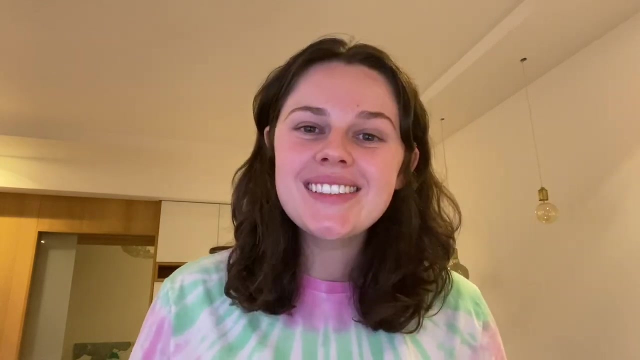 already dabbled in software. this is for people who absolutely have no clue and, i have to say, my most asked question in life is: what do you actually do? what does a software engineer even do? so today i'm answering that question. let's talk about how the ecosystem works. okay, the more that business goes online, 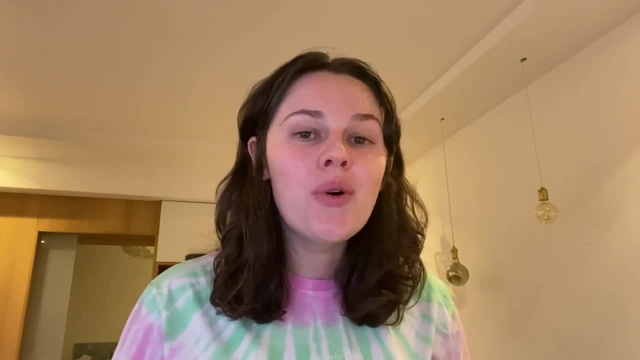 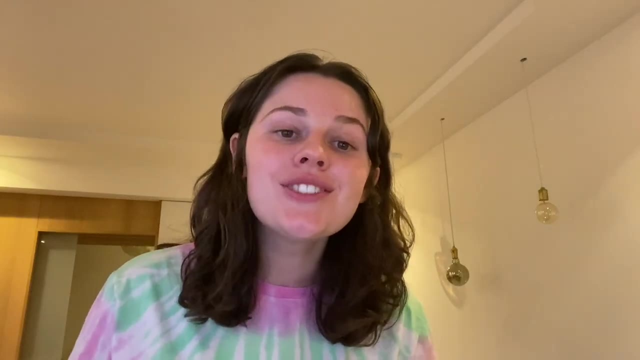 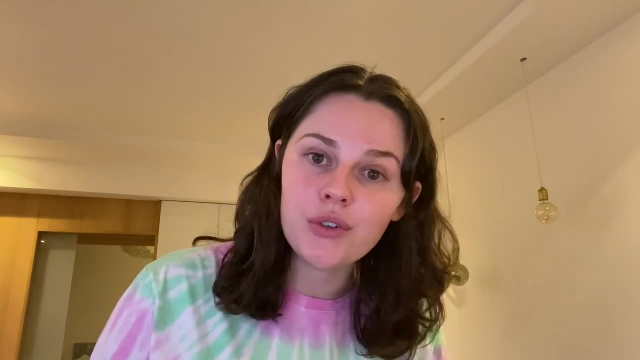 and everything we do in our day-to-day lives goes online, the more work we have to do. being able to do your online banking is not as simple as just whipping up a website. there's so much detailed management of your data, of having a nice user experience for you. 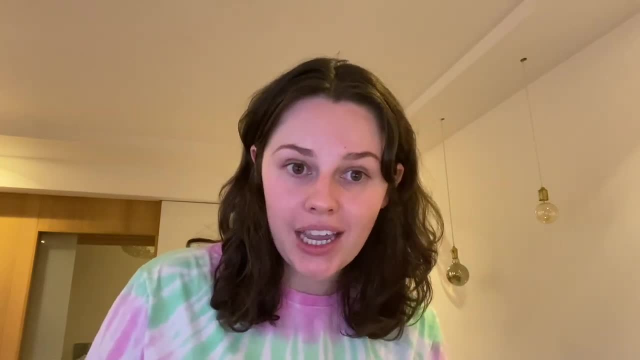 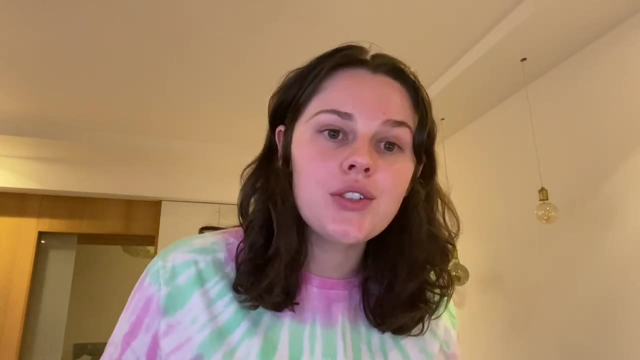 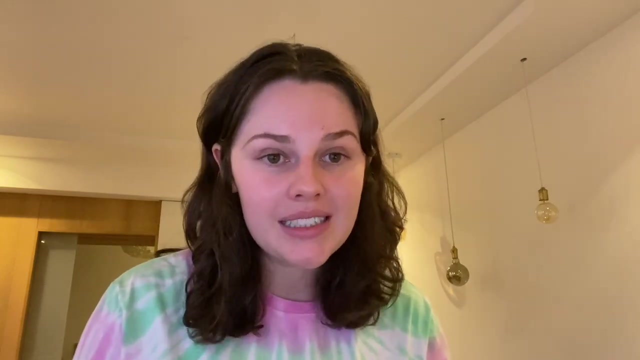 of security, of stability of the application, making sure when you log on you can log on, that the server doesn't crash, that you can access it when you need to. there's a lot that goes on, and the main reason i think that software engineers have jobs is because you, the customer, 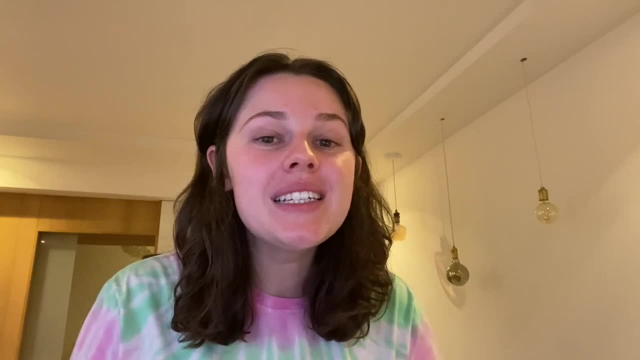 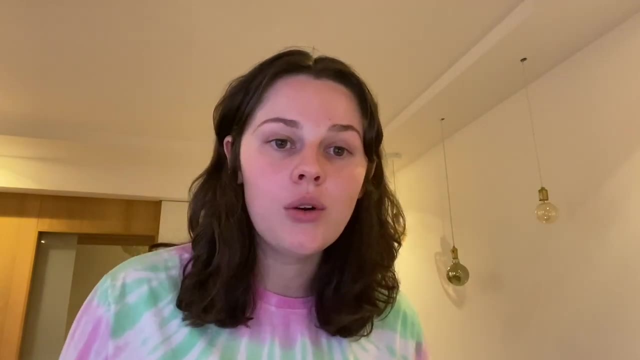 always want more, and that's fine. that's a great thing, but that means we need to do all of them to keep delivering more. the expectation becomes more for what you can do online, and we have to meet those expectations in order for the businesses to make money, to keep making money to. 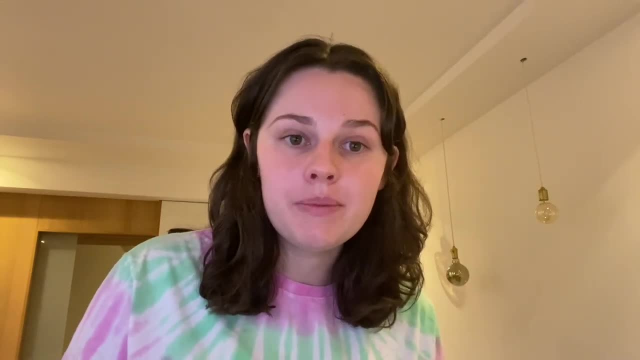 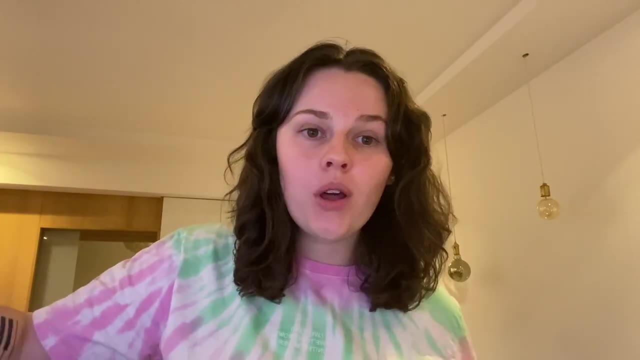 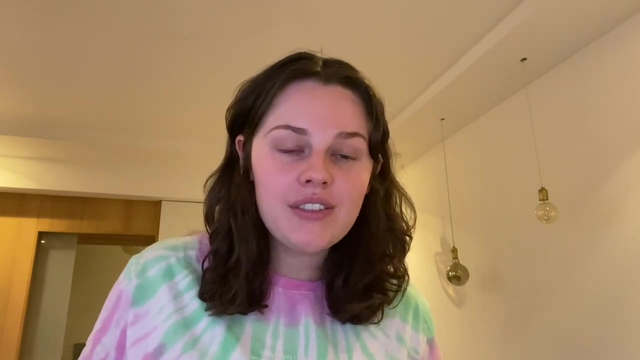 satisfy what you need from your online experience, and it doesn't start with us. it starts from senior management all the way through product design and it eventually ends up with us. so when you see a new feature, that's something that software engineers have spent possibly a month or two months building, and then they release it and then you can access it. 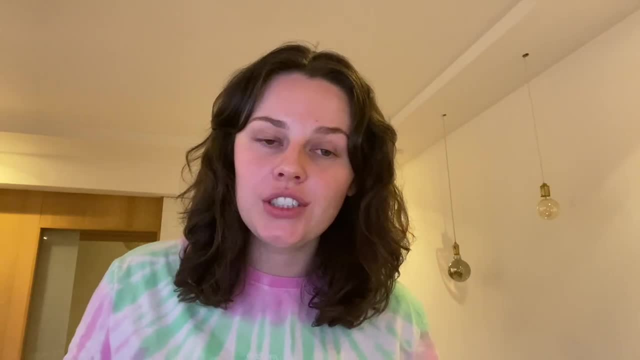 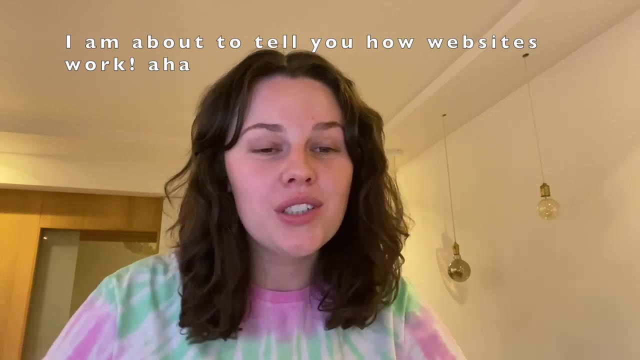 before i can tell you about the nitty-gritty of what we're actually doing day-to-day, you have to understand, i think, the most basic concept of all, which a lot of people don't. they don't get it or don't think about because they don't need to. so 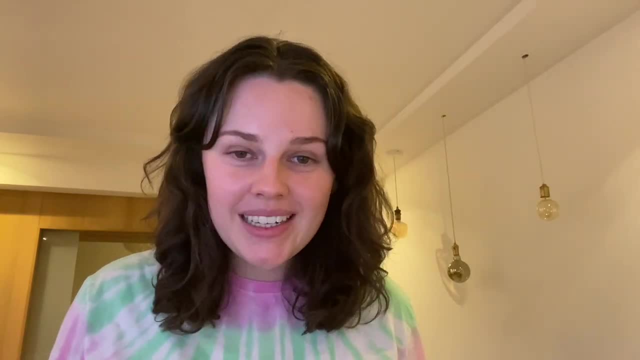 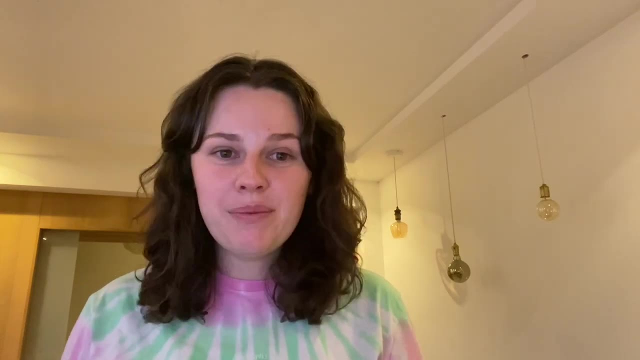 every time you go on a website, it's much more complicated and complex in functionality than i think we give it credit for upon first glance. we don't actually think about the journey we take on websites. we don't think about the fact that, okay, sure, i pressed the button or i went to 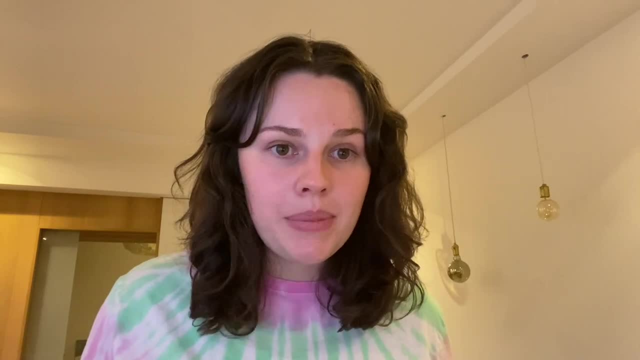 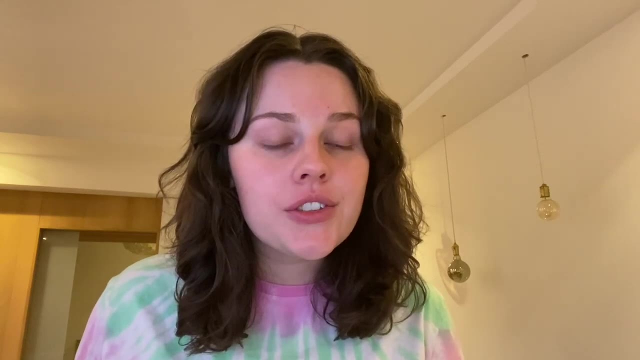 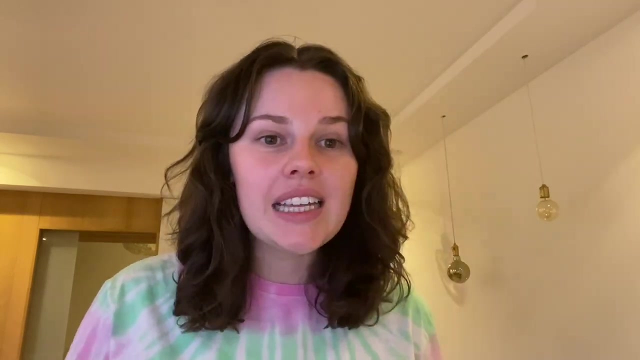 the next page. but we don't think about the fact that when i press that button, that sends a message to the server to redirect you to a different page. the server will receive your request from clicking that button and it will send you to that page if it's more advanced than that. 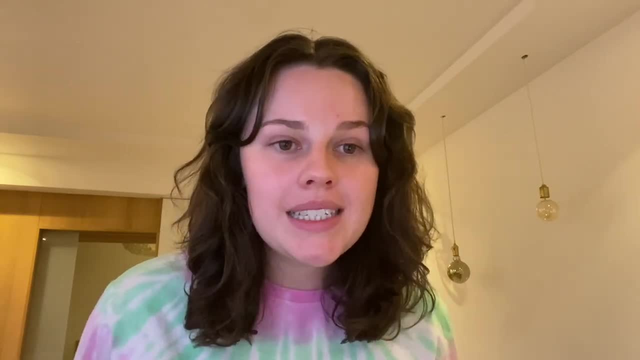 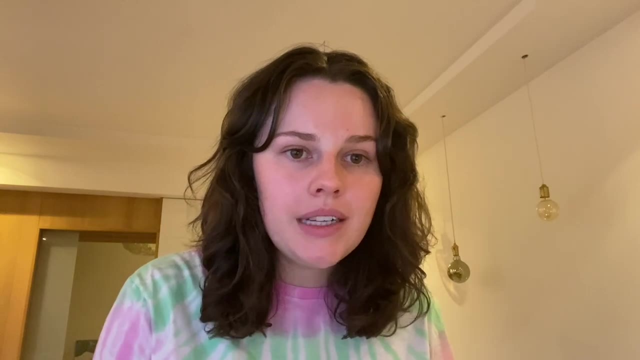 such as authorization. for example, maybe you want to see a page and you have to be logged into your account to see that page at some point in this flow- that when you press that button it will tell the server- hang on, we're just going to check that this person is logged. 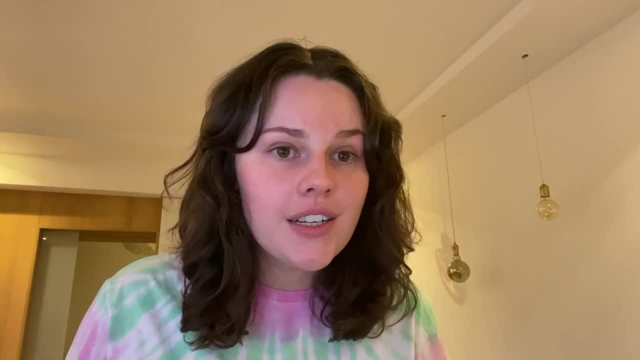 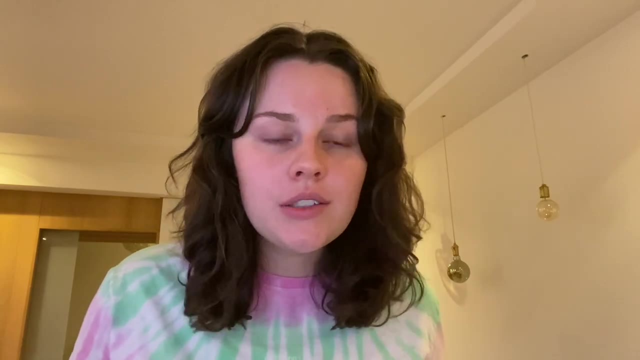 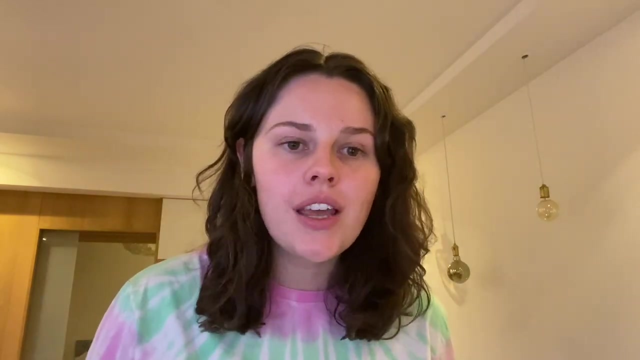 in and is allowed to see this page, and if that is true you will see that page. if that is not true, you will get an error message or you will be redirected to login. that's a simple example. another example is when you fill out a form, so say you type in your login. 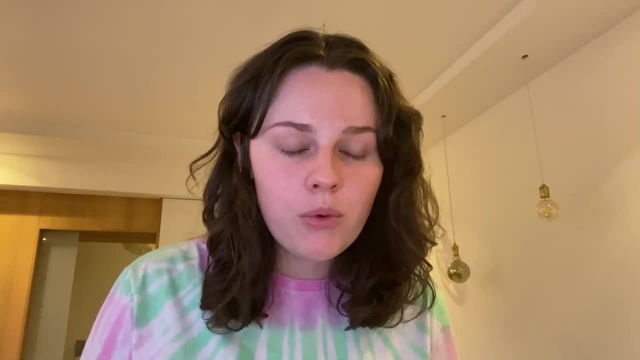 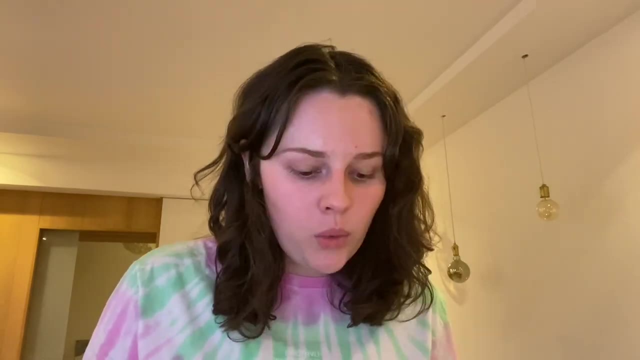 details. there's two fields. there's your- your username or email- and there's your password. so when you put your email in that and your password and you press login, what that button does is now: it's taking your input, it's sending it to the server, it's saying: use this. 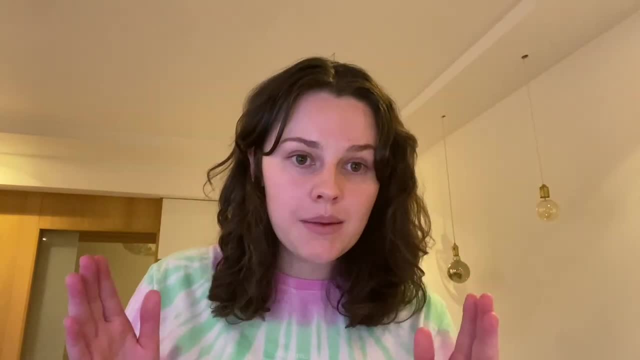 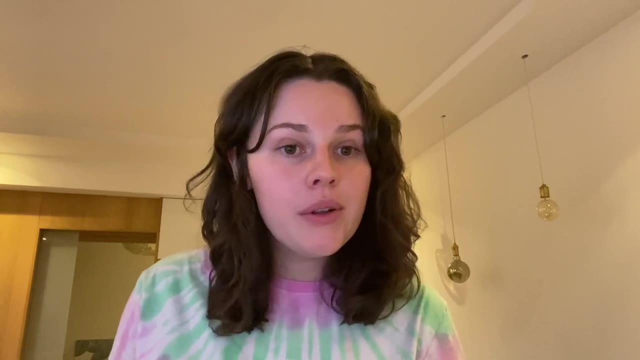 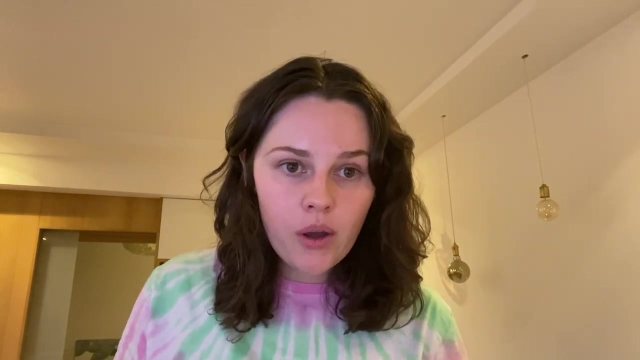 stream. we will call your email or your username a string. take this string of characters and find that in our user base. okay, we've found your account. now we want to check if the password you put in matches the password that we have. i want to jump in here and make a very important 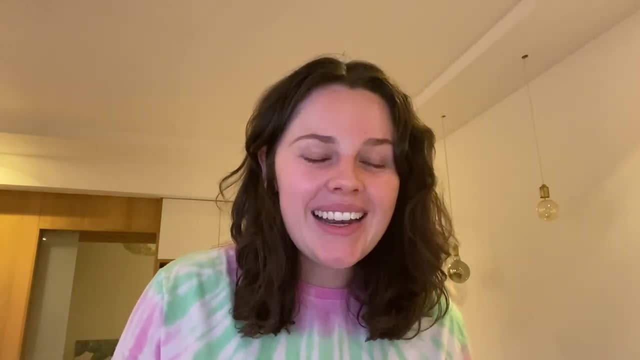 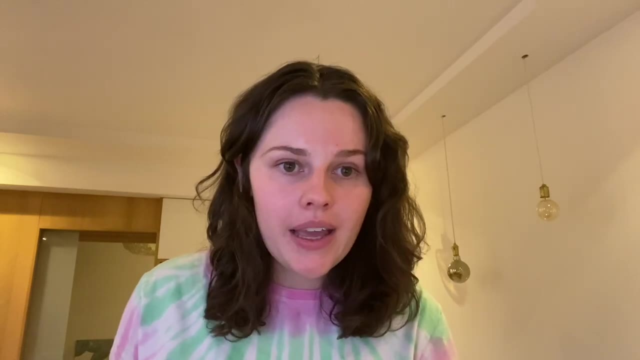 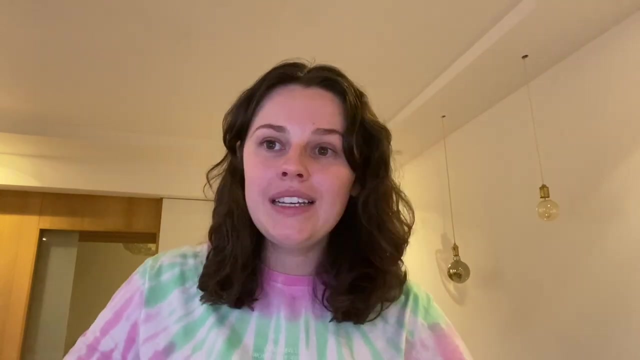 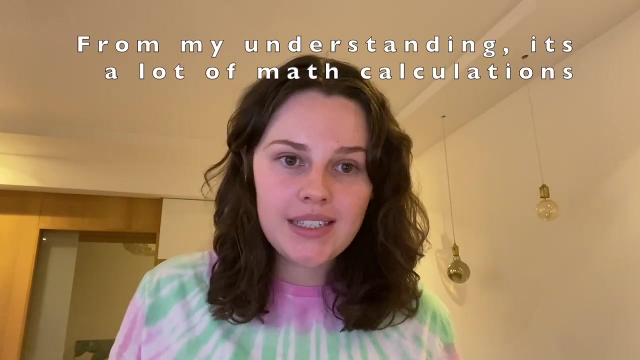 point about passwords. a good website, aka most websites, will encrypt your password. they can't see it. it's not saved in a database where we can see it and just copy and paste it. it's completely hidden behind a series of scrambled characters, numbers, symbols and there is a sort of decryption process from what you input to um. check if that matches the. 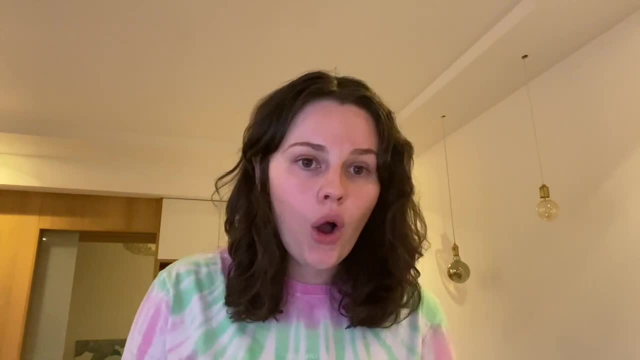 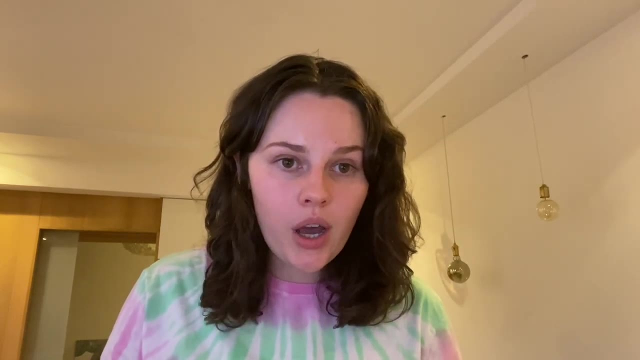 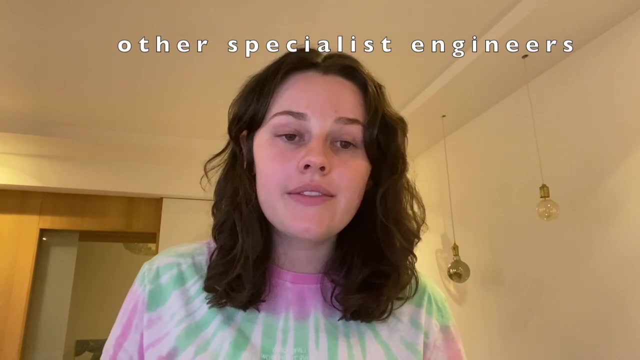 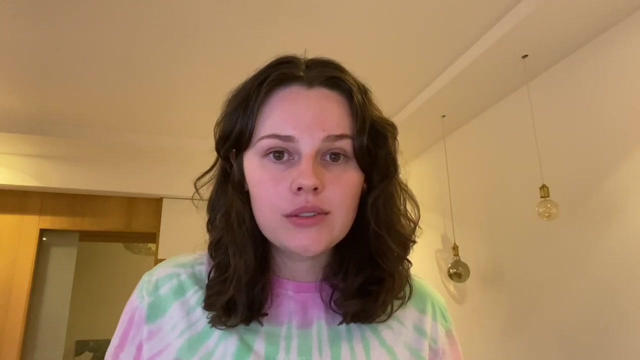 the encrypted password that is saved. but that whole process of comparing your password input to the encrypted saved password, that whole process of of figuring that out, is handled by typically an external provider that has invested a lot of money into ensuring very, very strong encryption. so that is that's what that looks like. we don't save your password in our database because that. 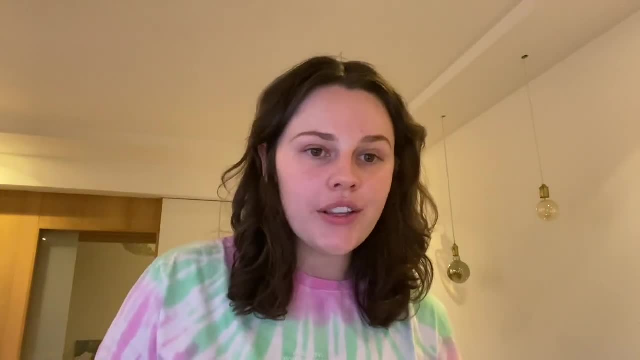 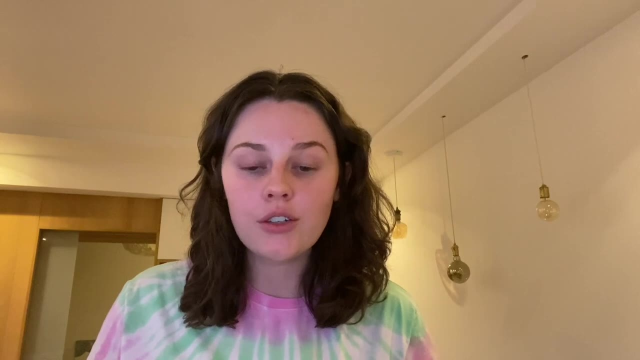 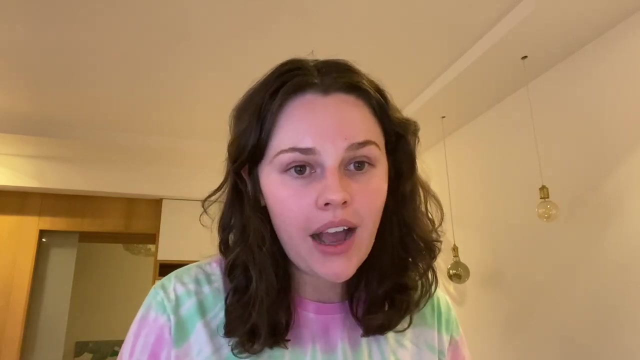 will be very high risk. and so, engineers, we have to tell the computer, take this information, run this uh encrypted comparison process and then return back to you a positive or a negative outcome. if it's a positive outcome, you get to log in and then so, with the positive outcome we show, we say 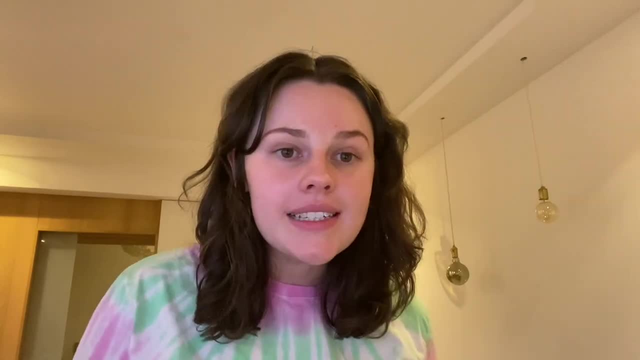 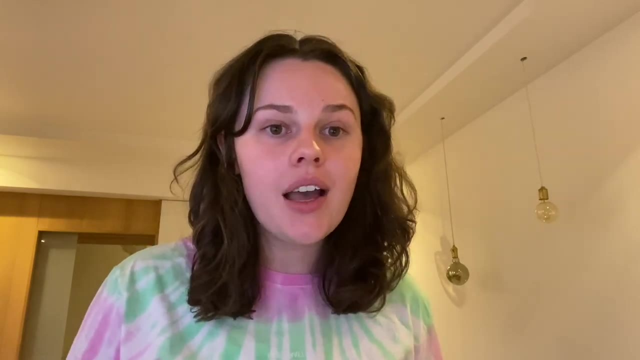 okay, here is the page that you want to see. if it is a negative outcome, then we ask you to try again, or maybe your account will be locked if it's been done a number of times. so there's another thing an engineer might do, or perhaps the password. so 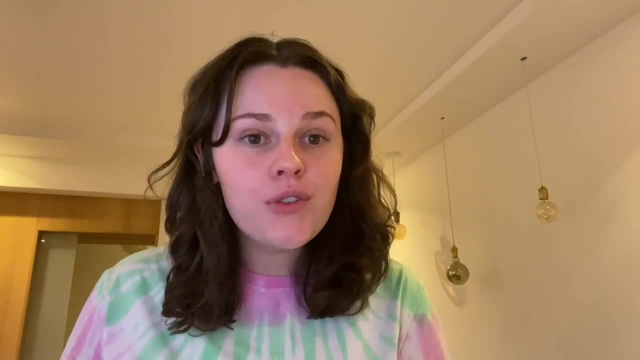 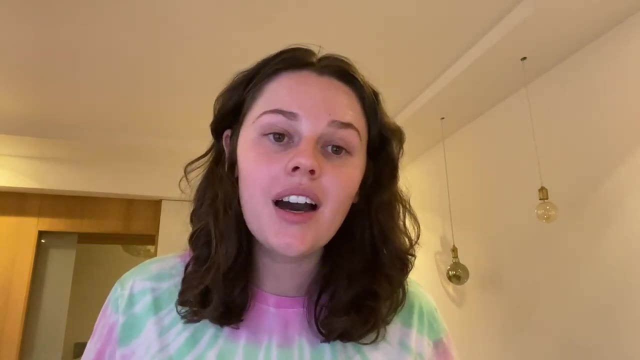 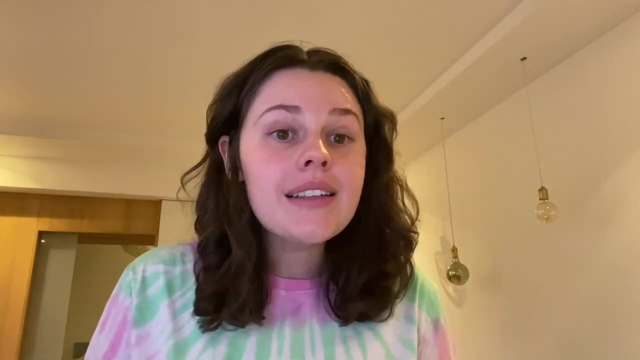 software would do is they would say: if you have attempted this five times and you've not been successful, we will lock your accounts. those are a few examples of the kind of logic we need to write, and it's all very much based around true, false success, error, things like that it can often be. 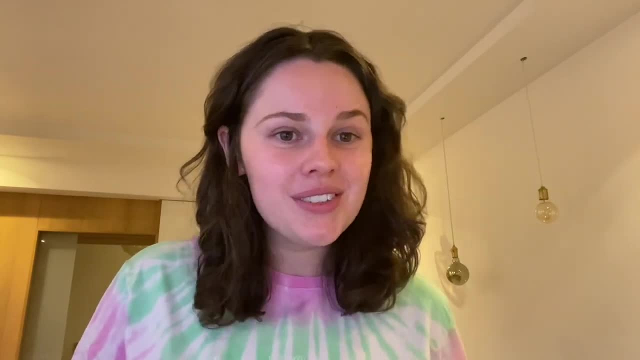 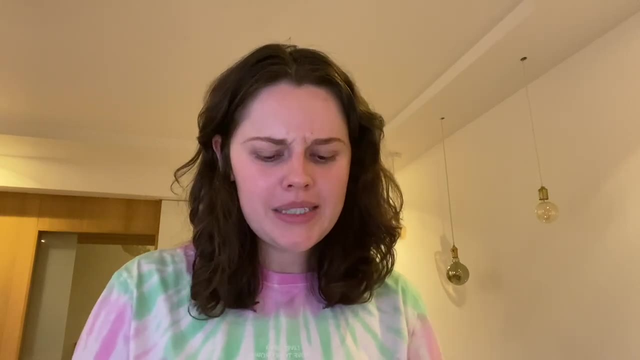 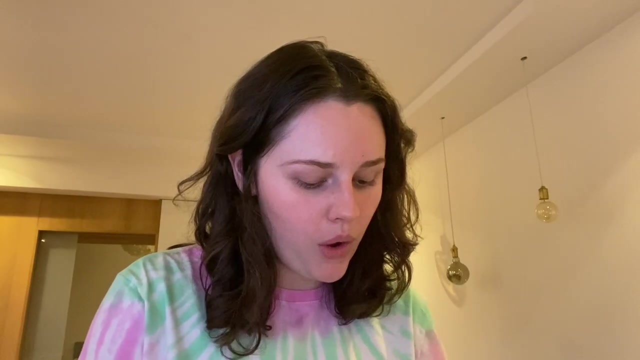 like one of those quizzes you would do when you're like a teenager in like female sort of focused magazines. you'd have this little like map and you would start with the first bubble and the first bubble would say: do you have brown hair? yes or no? and if you, yes, and then it would go: okay, do you like music, whatever, yes or no? and you say: 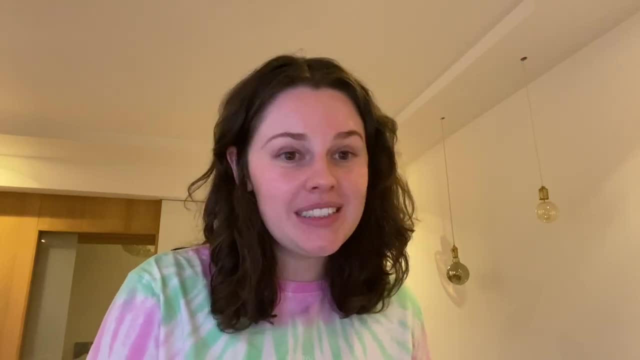 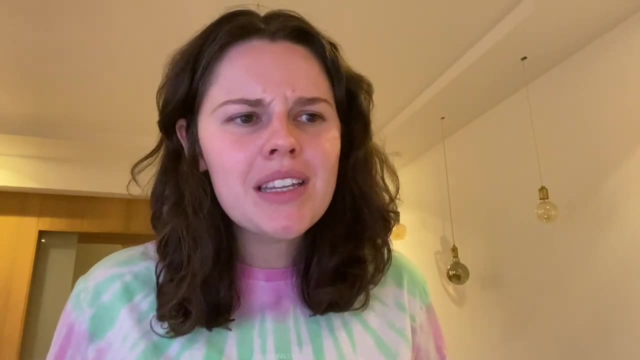 okay, no, do you like sport, yes or no? and you go yes, and it sort of takes you down this tree of options until and then it tells you like something at the end, or you're a sagittarius or something like something dumb. you know what i mean in that example: it's dumb, but 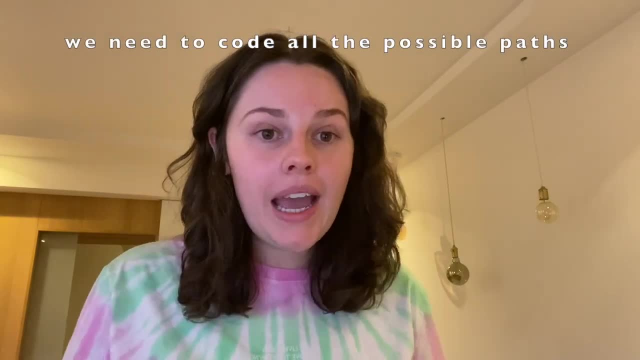 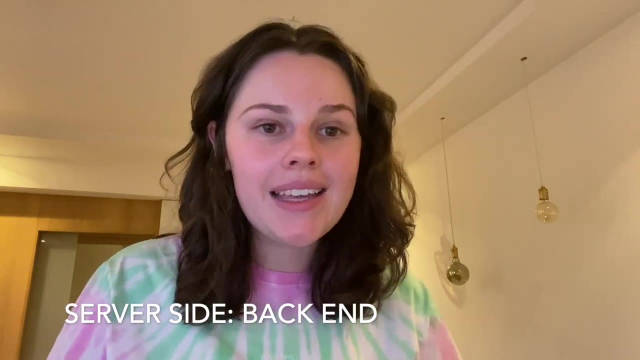 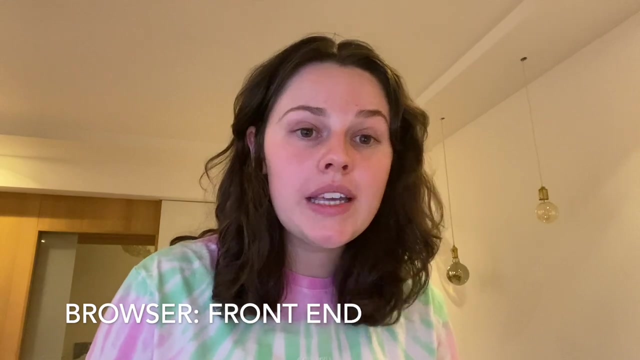 we're getting kind of like a sort of a sort of path we have to create for you to navigate the internet. the examples I've given you are very much back-end engineering style examples. however, front-end side of that is actually it's okay. you hit submit on the button of your username. 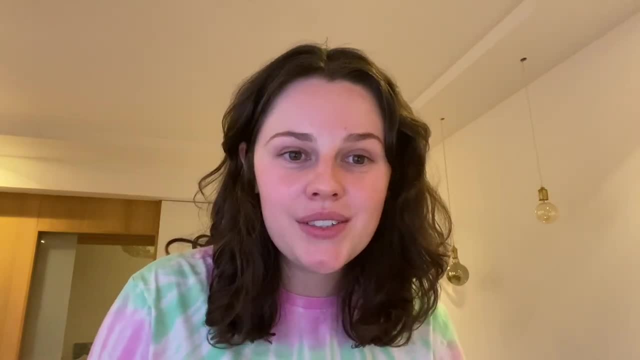 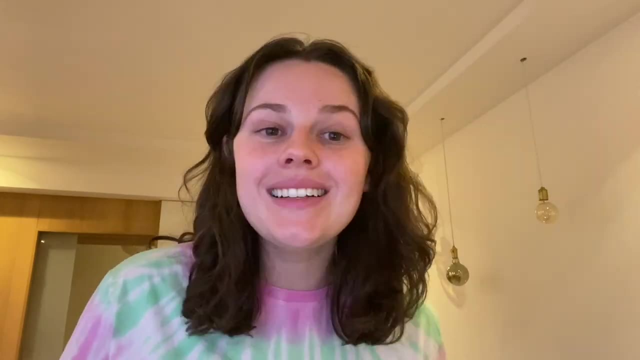 and your password. that sends to the server. so that's a front-end task, but as a general rule, everything you see on the browser is considered front-end with call-� manipulation is typically the back end. However, it's not black and white like that. It completely. 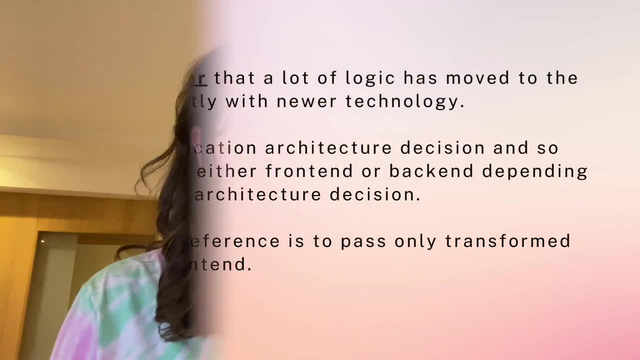 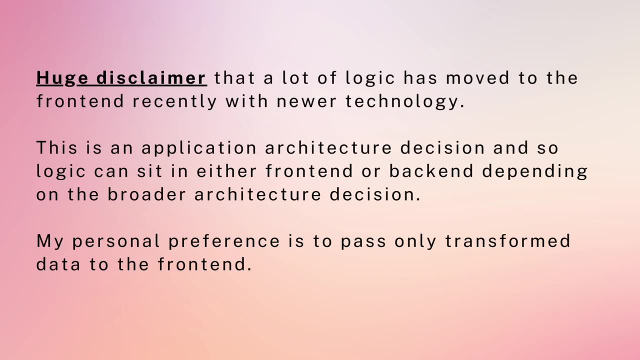 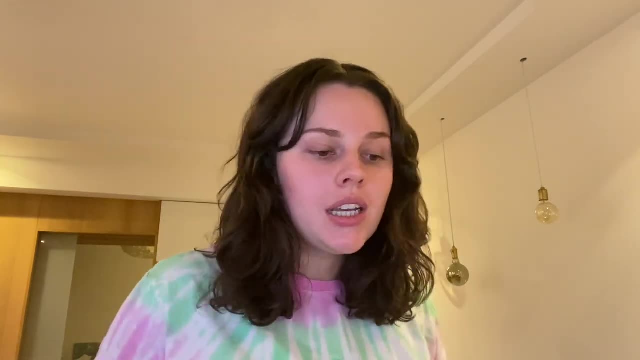 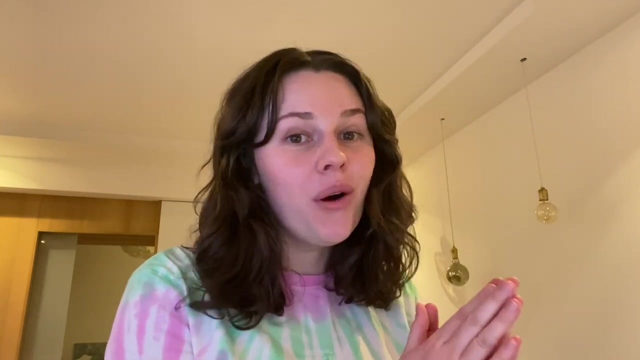 depends on the architecture of that website When it comes to actual day-to-day tasks. for a very simple basic explanation, there will be something we call a ticket. It will have requirements for a section of a feature- very unlikely to be the whole feature- and then I think I'm going to have 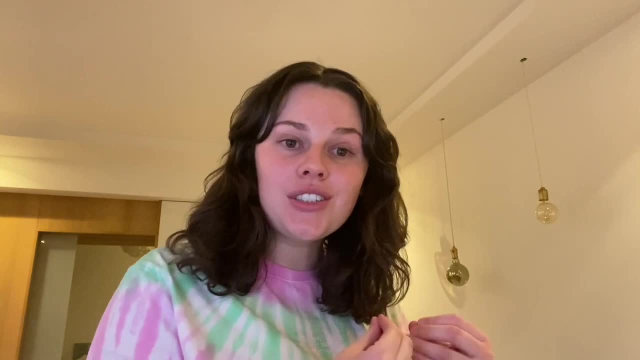 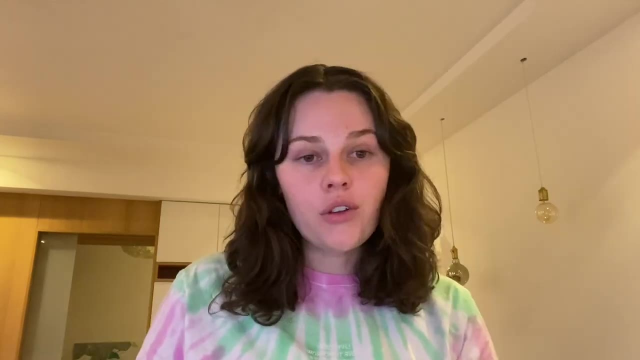 some opinions on workflow there. So it's a section of a feature that your whole team is working on and you would pick up that ticket. you would assign it to yourself. you've got the code base. you've got the local version of the website. It's like a copy of what you're seeing on the internet. 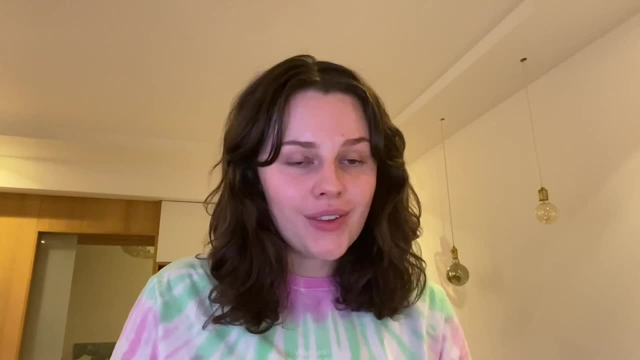 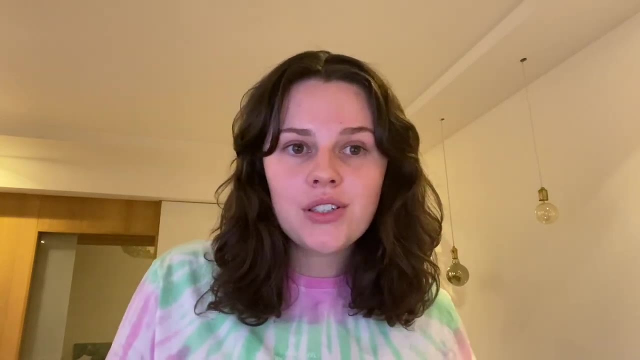 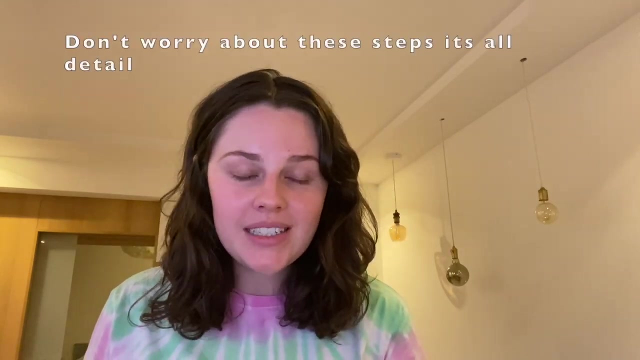 but it's on our computer. With this copy of the website, you see, we code a solution and that could take anywhere between less than an hour up until a week- perhaps That's completely dependent on your team's workflow- And then to skip a number of steps when it's all been approved by teammates. it's 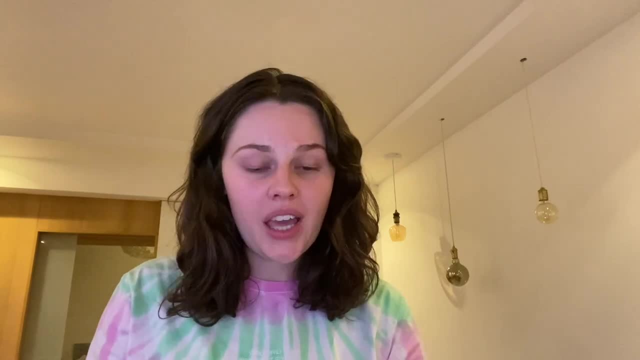 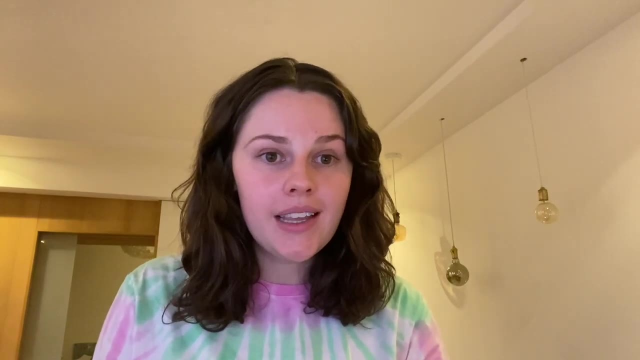 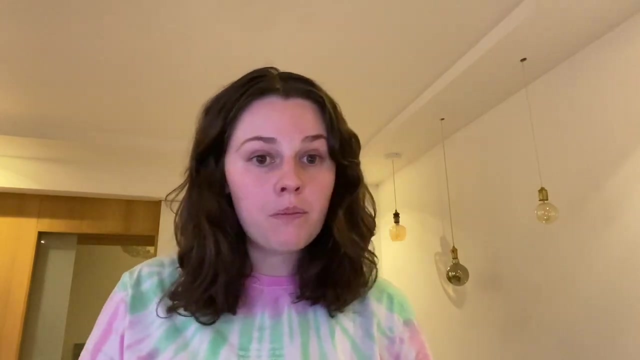 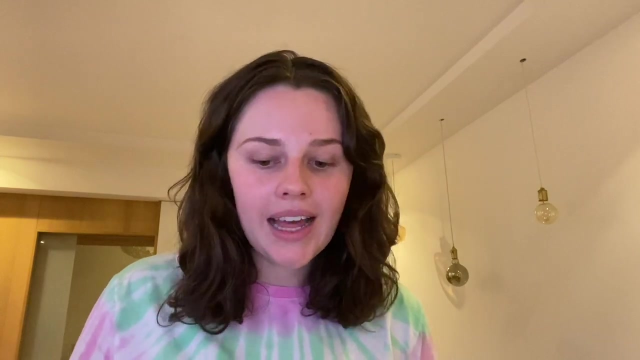 been tested. it's working. then you can merge it into the version of code that is serving the website. you see, And that's why one day you can literally hit refresh and suddenly it's there, because when that finishes merging into what you see, it will show live on production. we call it production, So that is how we create these changes. 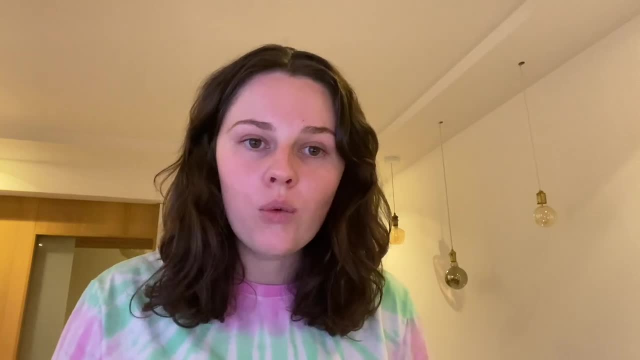 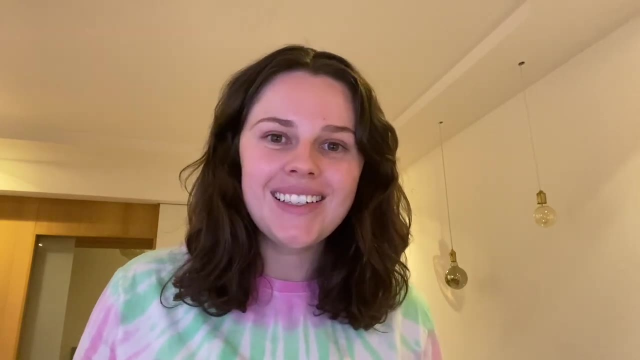 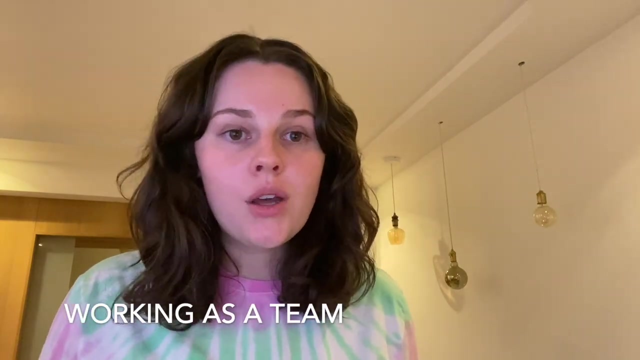 update the website again and again and really like a very good workflow is for that to be happening pretty much every day. Small little changes are happening every day to these websites that you're browsing on And you don't even realise, So I think it's very cool. It is also very common outside of just coding that a software engineer will spend time in. 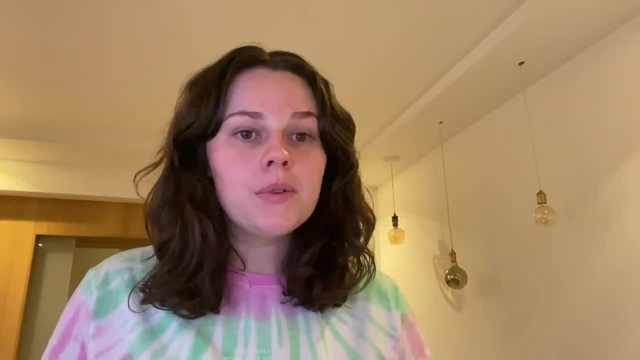 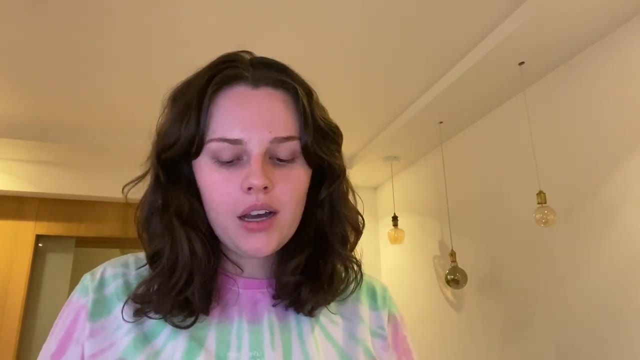 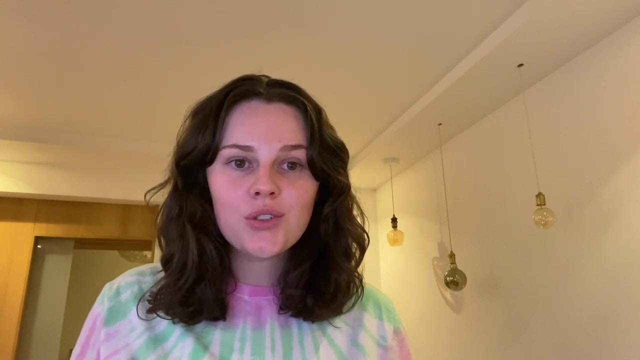 meetings with teammates or other engineers- engineers or product people- discussing requirements, discussing, like the feature that needs to be made, how it will be made, broader decisions around architecture, and when you write these solutions. there is a number of ways to solve the problem, and so a big part of being a software engineer. 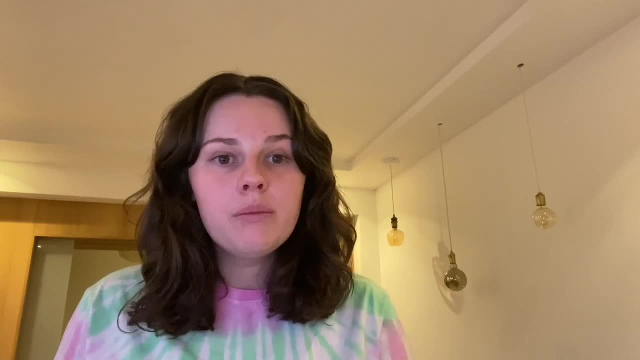 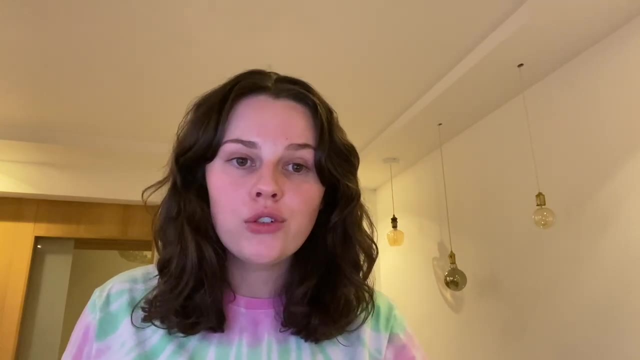 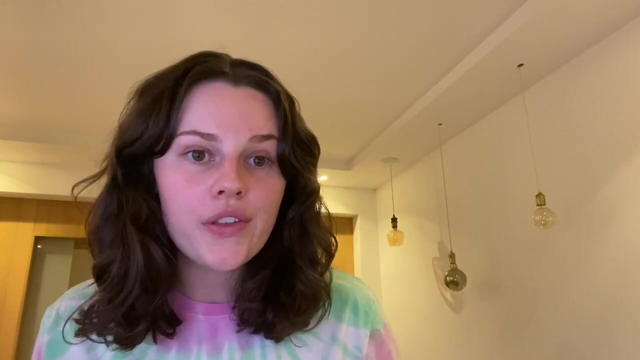 and the skills and knowledge you need to have is: what is the best way in this situation to solve that problem, given your time constraints, given the- uh, long-term implication that your code will have on the, on the application itself, and sometimes you have to ask: is it worth it, am i adding? 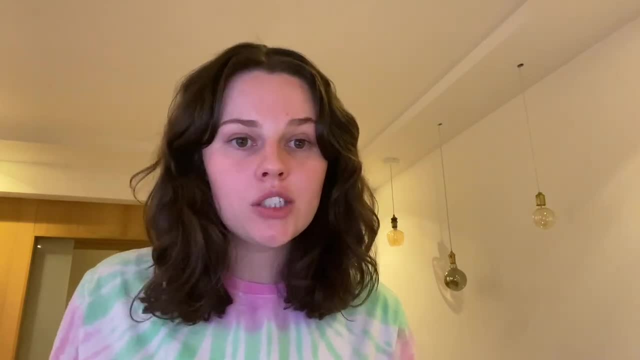 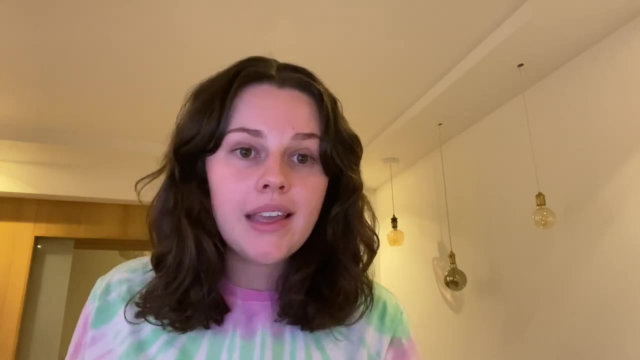 something to very old code that's no longer in the architecture we want. do i spend a lot of time making it like the new one or do i just? it's a small thing, i would just make it fit for now and then sort of the next project might be breaking that part of the code base out or rewriting it. 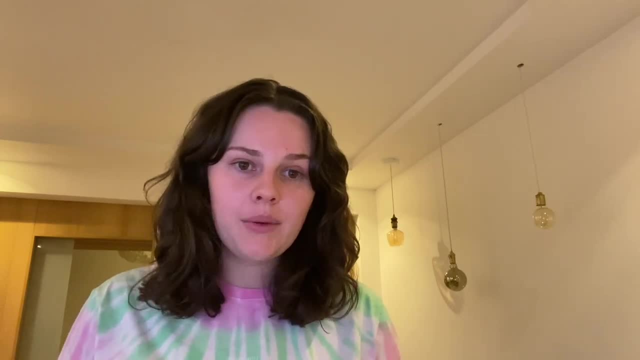 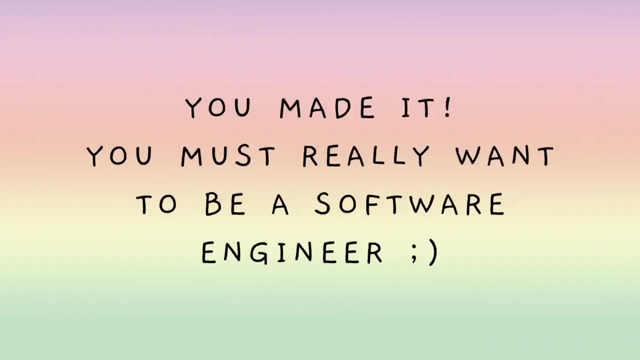 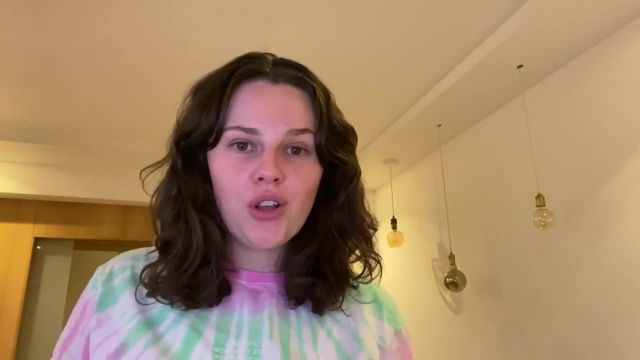 in the new way that you want it, a lot of the understanding we need to have. it goes far beyond languages and it goes very much into this architecture space. so, anyway, i am sure that was a huge information overload for you, but if you manage to make it, 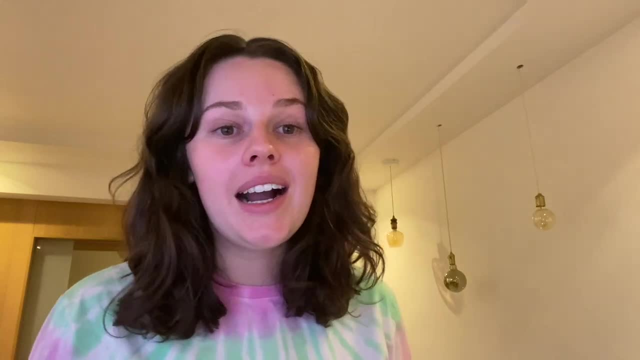 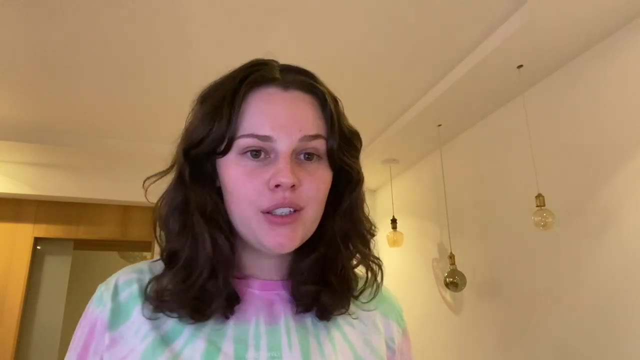 through. i really hope that gives you a very simplified idea about what we actually do in our day. not just did i pour a cup of tea and i'm like, oh my god, i can't do this, i can't do this, play lo-fi music. actually, what we are doing between the hours of nine to five. 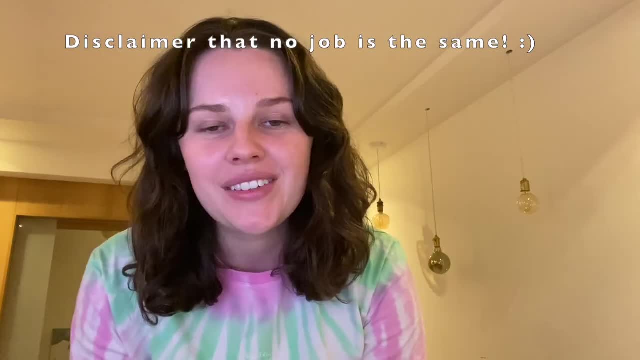 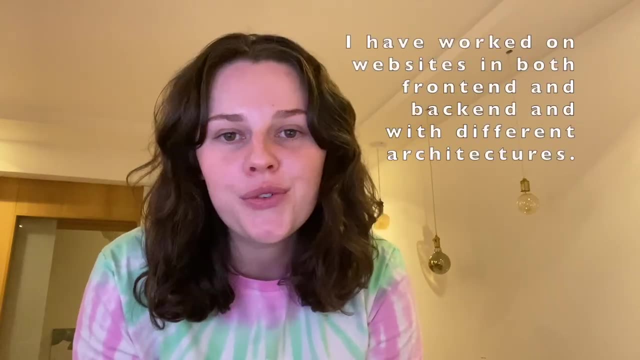 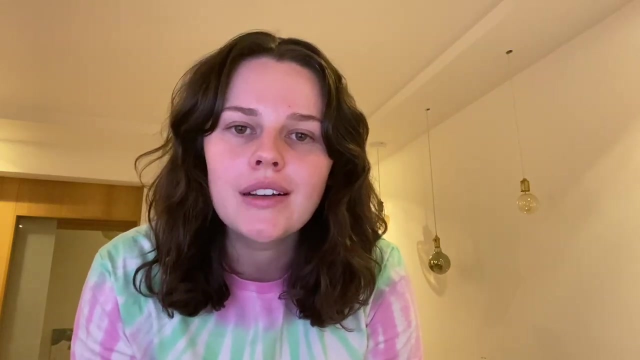 Now I do want to say that the example that I've given you is not the same for every software engineer, but that has been the consistent trend across the few software engineering jobs I've had, and so I think it's a very, very good insight. If anyone's doing it very differently, that would be.